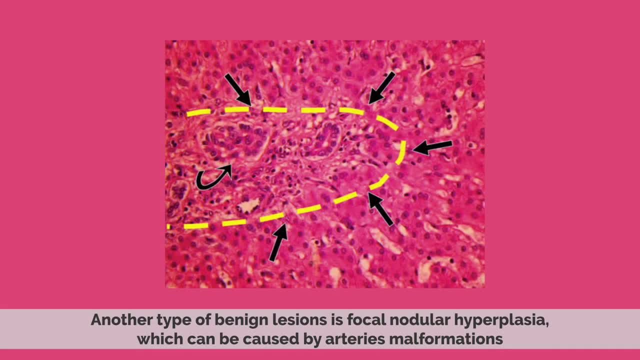 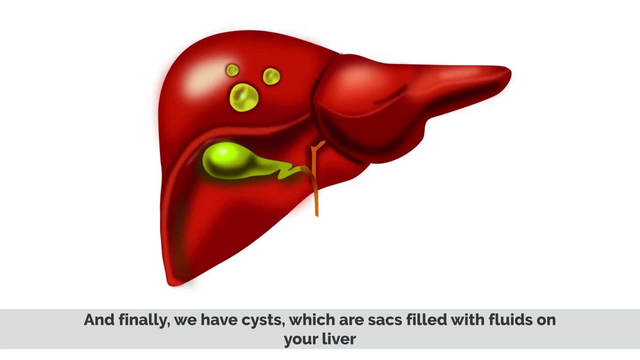 that cause a tumor on the liver. Another type of benign lesions is focal nodular hyperplasia, which can be caused by arteries malformations And finally, we have cysts, which are sacs filled with fluids on the liver. Malignant liver lesions, on the other hand, are usually cancerous and can 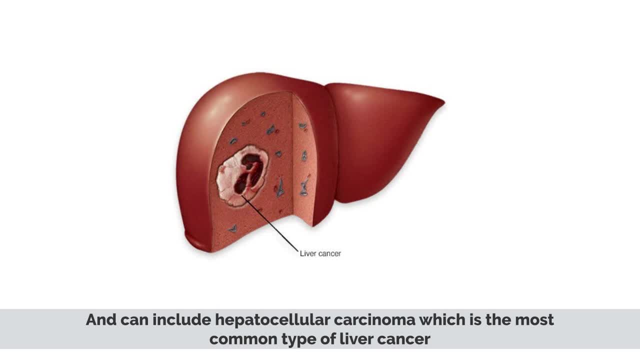 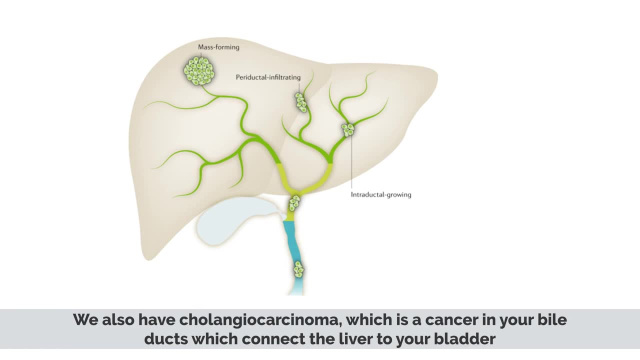 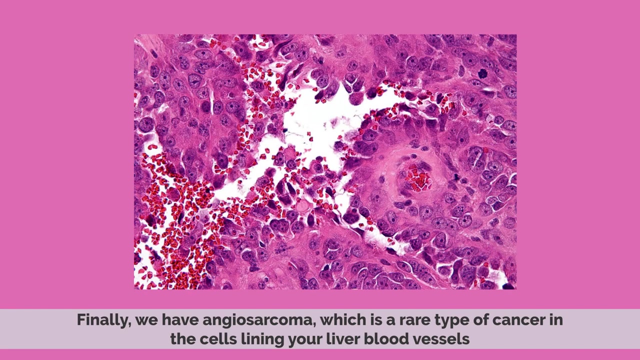 include hepatocellular carcinoma, which is the most common type of liver cancer, and it is a self-threatening condition. We also have cholangia carcinoma, which is a cancer in your bile ducts which connect the liver to your bladder. Finally, we have angiosarcoma, which is a rare type of cancer in the cells lining of your liver. 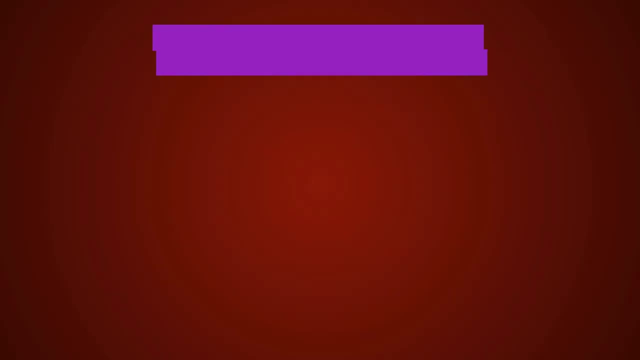 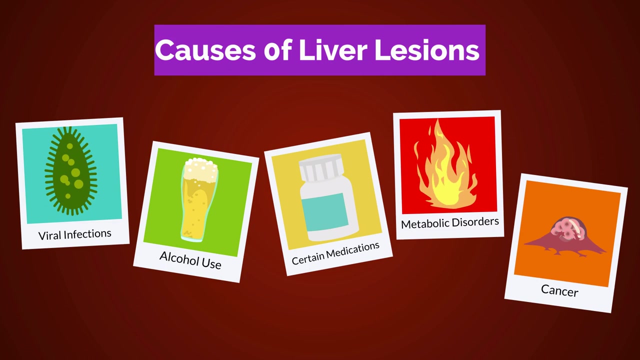 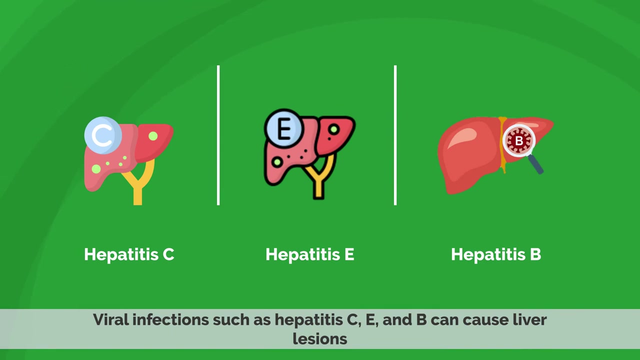 blood vessels. Causes of liver lesions. There are a variety of causes of liver lesions, including viral infections, alcohol use, certain medications, metabolic disorders and cancer. Viral infections such as hepatitis C, E and B can cause liver lesions. Long-term alcohol use. 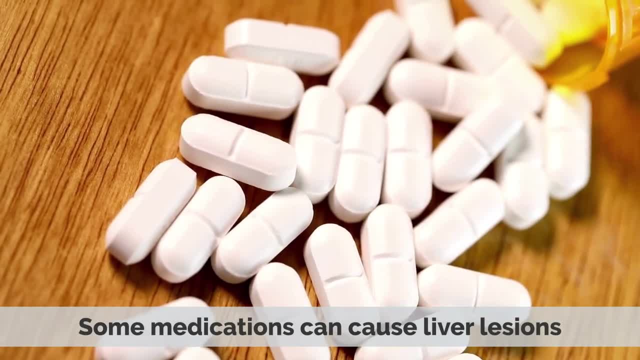 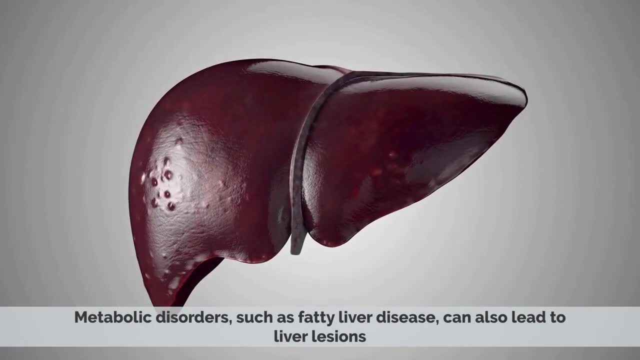 can lead to cirrhosis and liver lesions. Some medications such as hepatitis C, E and B can cause liver lesions, including certain birth control pills, antibiotics and statins. Metabolic disorders such as fatty liver disease can also lead to liver lesions. 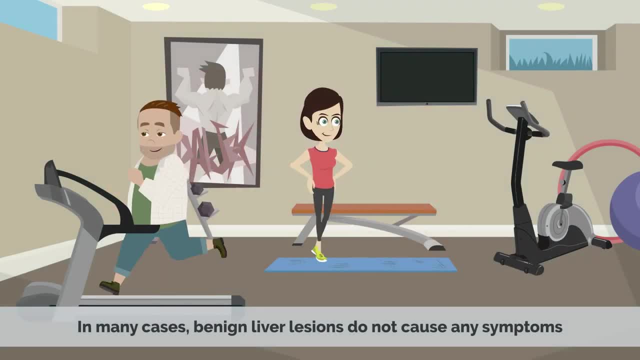 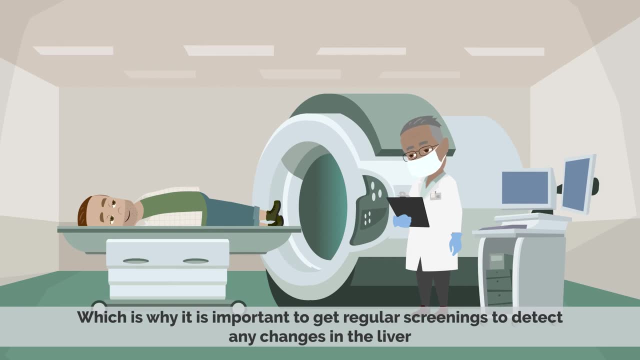 Symptoms of liver lesions. In many cases, benign liver lesions do not cause any symptoms, which is why it is important to get regular screenings to detect any changes in the liver. But if the liver lesions are cancerous and they get big and do cause symptoms, 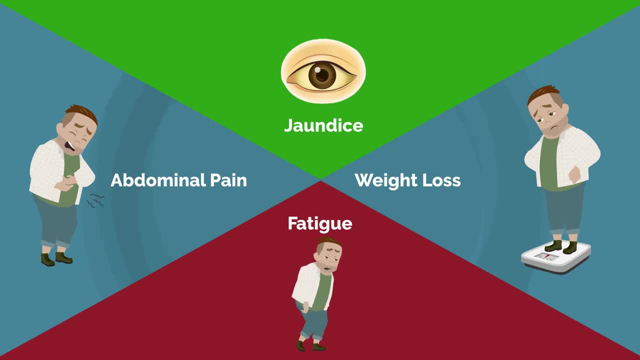 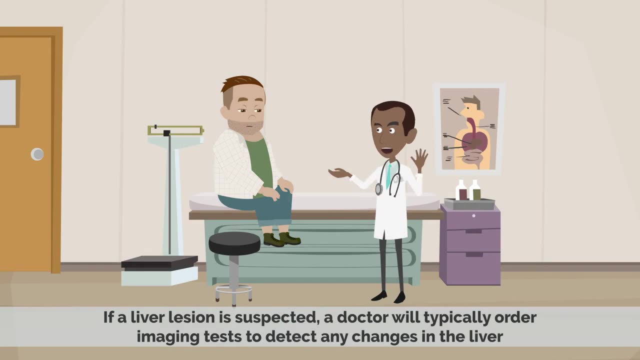 they can include abdominal pain, Weight loss, jaundice and fatigue. Diagnosis of liver lesions: If a liver lesion is suspected, a doctor will typically order imaging tests to detect any changes in the liver. These tests can include an abdominal ultrasound. 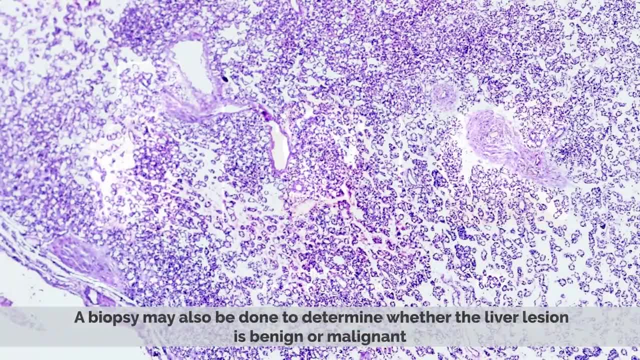 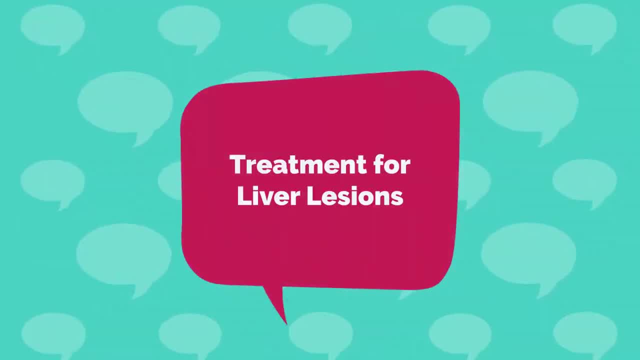 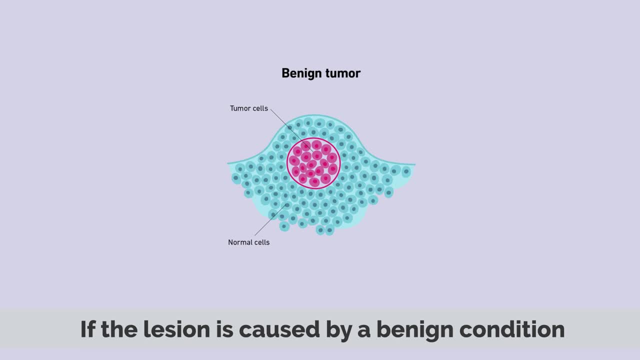 computed tomography, CT scan or MRI. A biopsy may also be done to determine whether the liver lesion is benign or malignant. Treatment for liver lesions. The treatment for liver lesions depends on the underlying cause. If the liver lesion is caused by a benign condition, then it will typically not require. 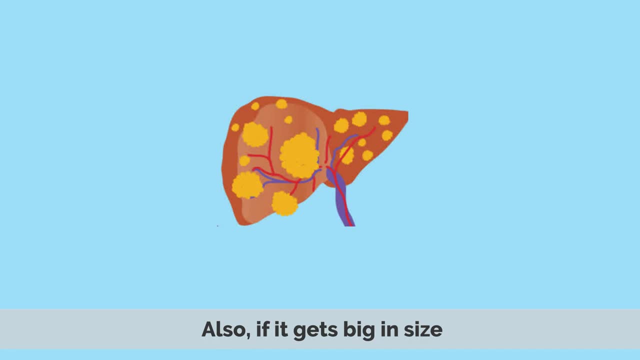 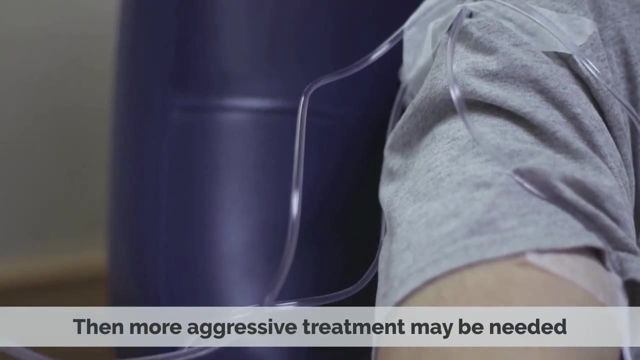 any treatment. Also, if it gets big in size, it may be surgically removed. However, if the liver lesion is caused by cancer, then more aggressive treatment may be needed. Treatment may include surgery to remove the lesion, as well as chemotherapy.